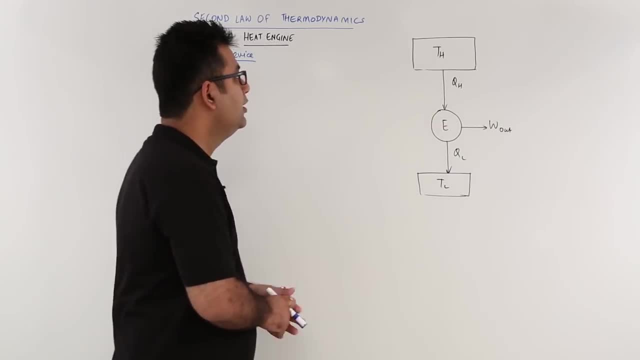 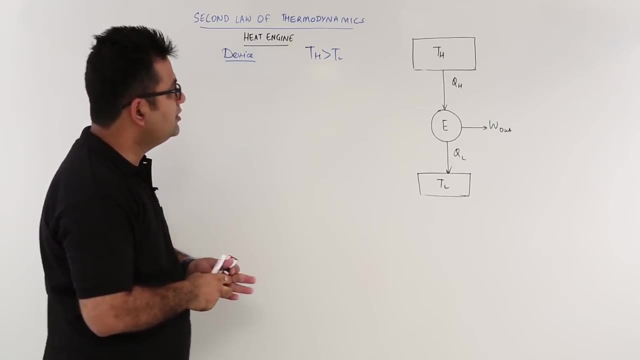 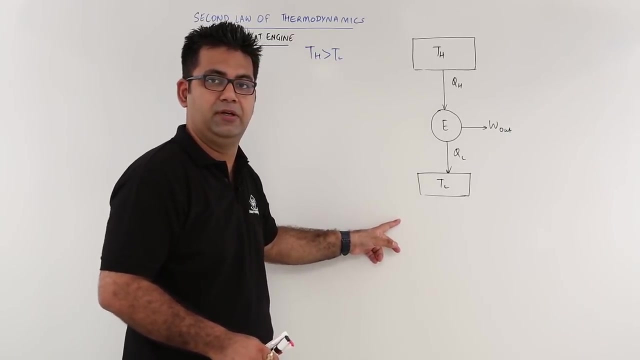 So these are two temperature reservoirs, TH and TL, So where we assume that TH is always higher as compared to TL. So because this temperature is higher, the spontaneous flow of heat is always from a high temperature to a low temperature, So your heat will start flowing from this to this. 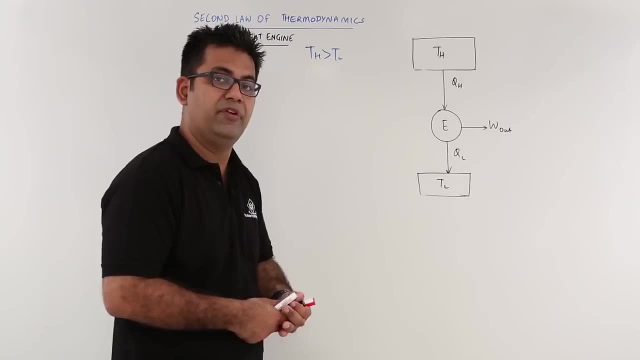 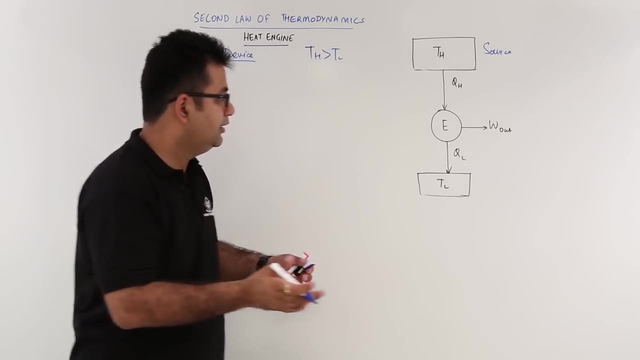 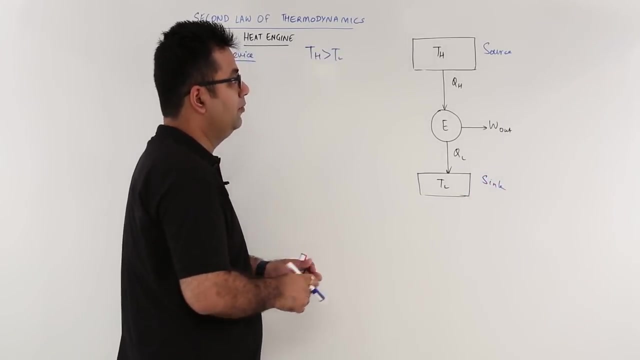 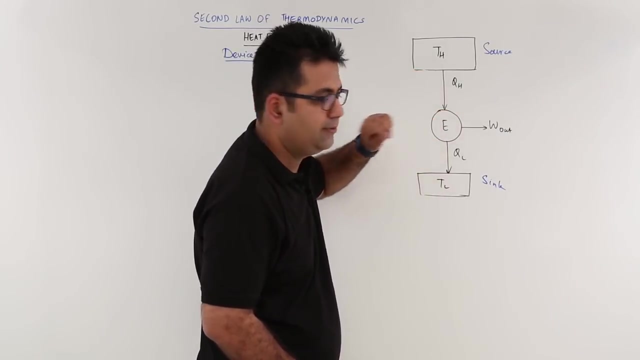 So the reservoir from which the heat starts to flow is also called the heat engine, And this is where you are rejecting your heat, So this becomes your heat sink. Now from heat source. this heat engine absorbs some energy in the form of heat. 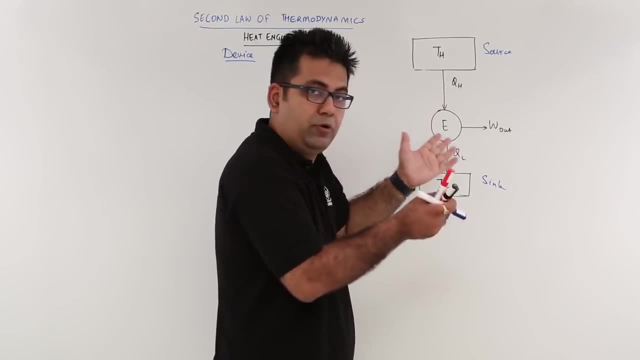 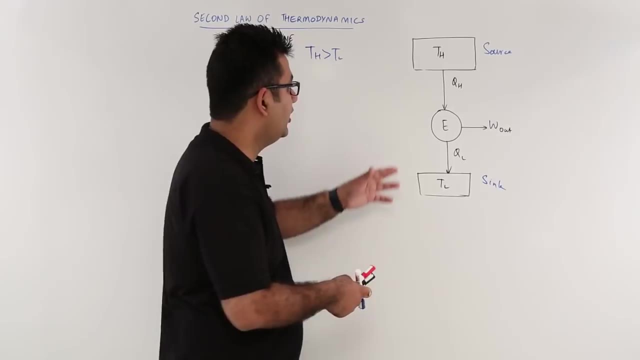 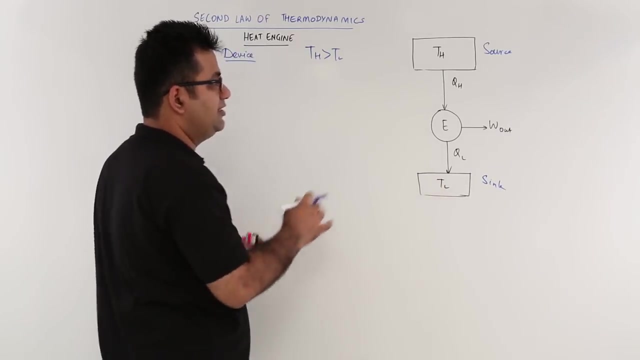 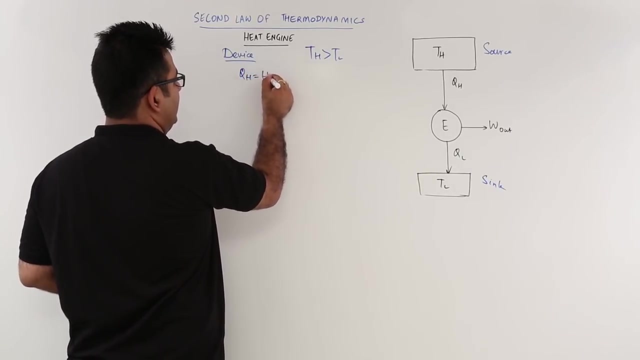 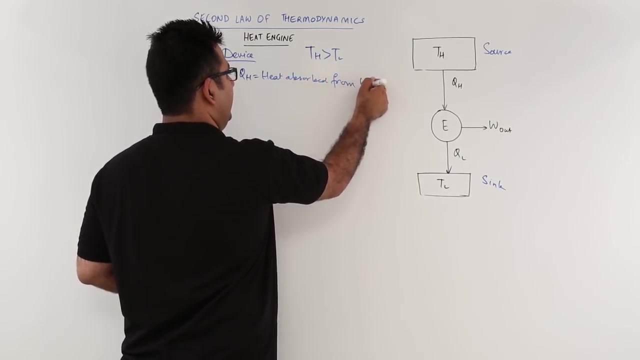 It utilizes some amount of that heat energy and gives out some work output, And whatever part is left which is not converted into work output is thrown out. So this is a very, very simplistic schematic of a heat engine. So if you talk about QH, this is the heat absorbed from heat source. 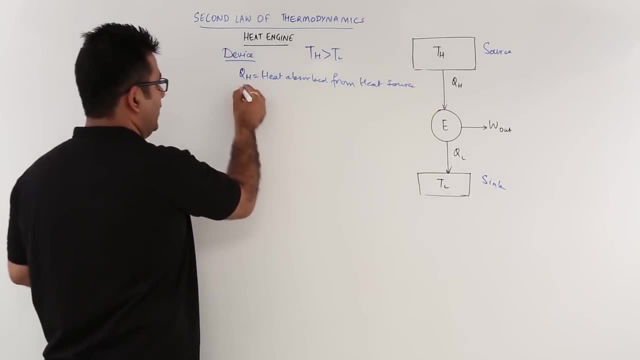 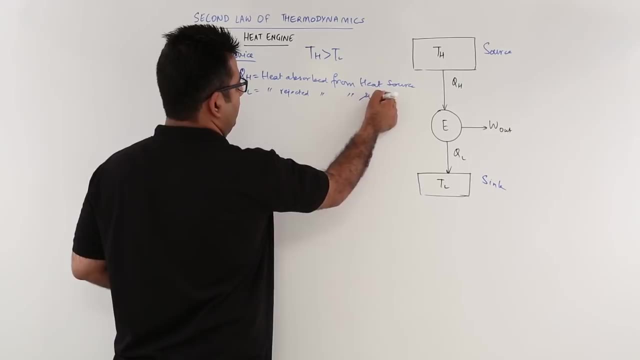 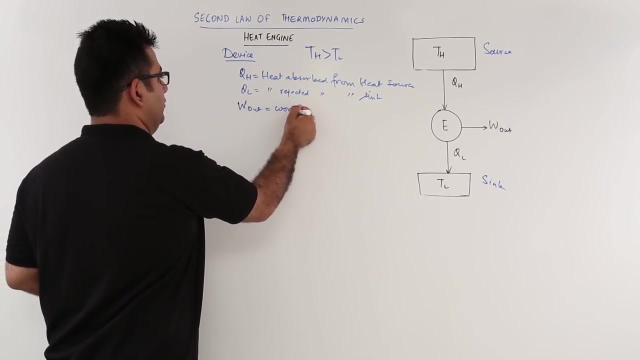 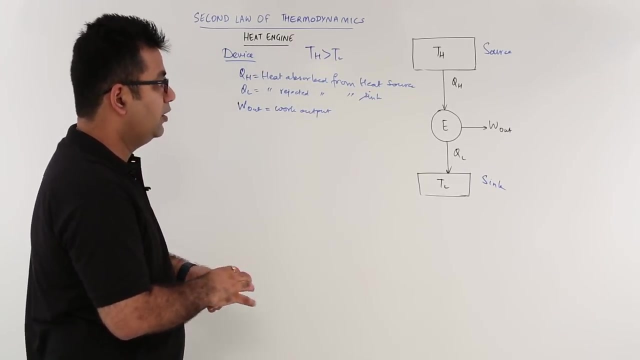 QL is the heat rejected from heat sink. Now work out. this is the work output. So if you get the relationship between these three quantities- QH, QL and W- out, look at this. This is the system that we will be discussing about. 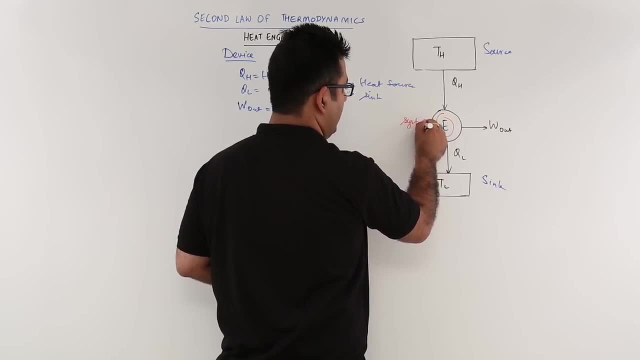 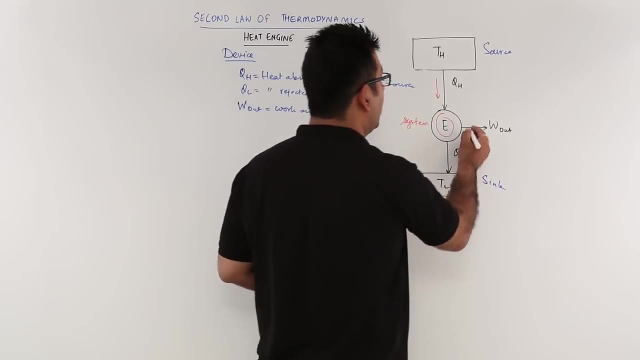 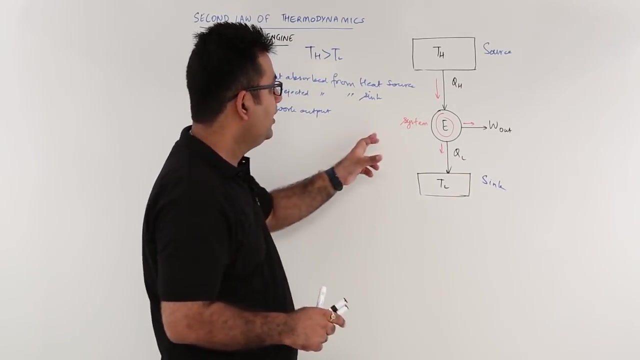 So this is the system. You have something coming into the system, So this is input to the system, And there are two things which are going out. This is going out and this is going out. So to maintain the energy balance of this system, the input energy should be equal to the outgoing energy. 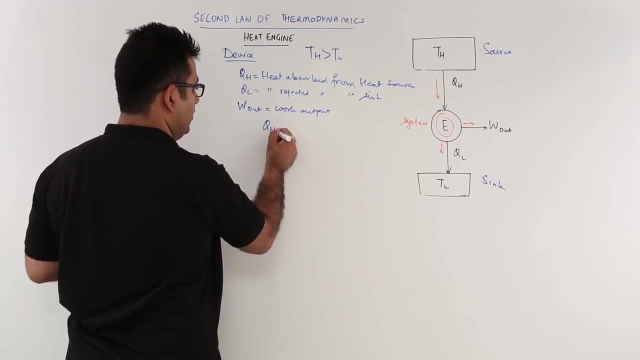 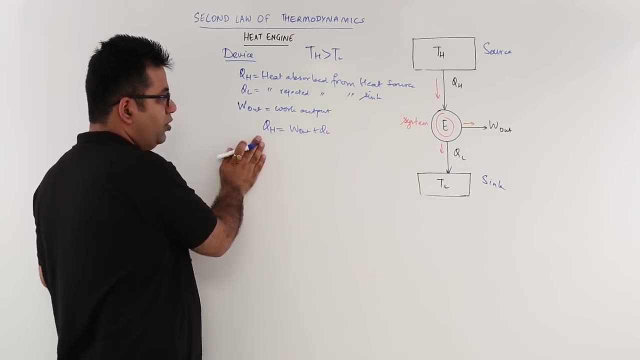 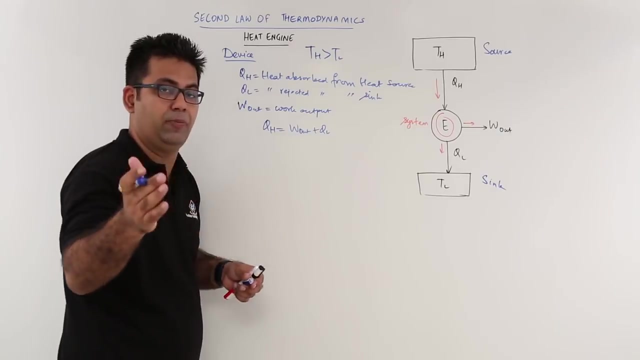 So you will be equating: QH is equal to W out plus QL, So input energy is always higher as compared to the output work. You can never have QL to be zero. This is an inaccessible topic we will be discussing about. 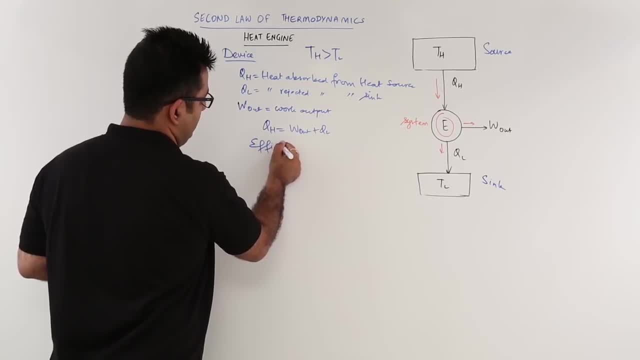 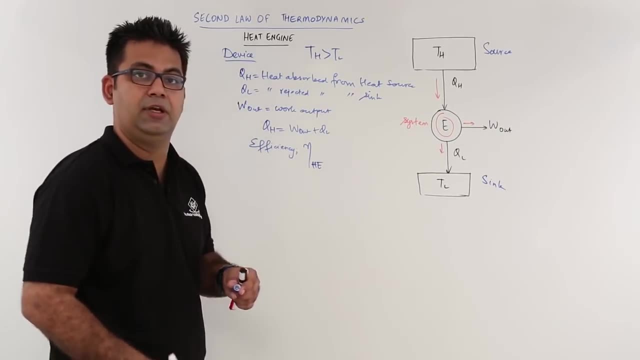 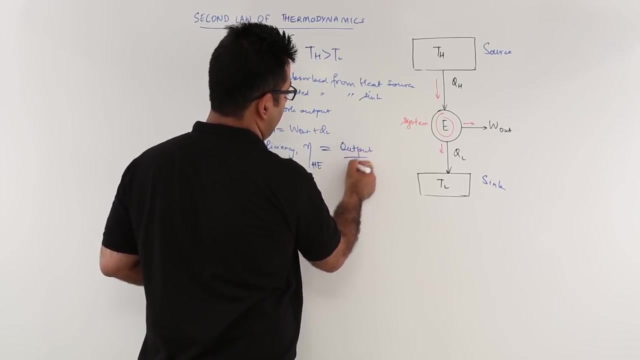 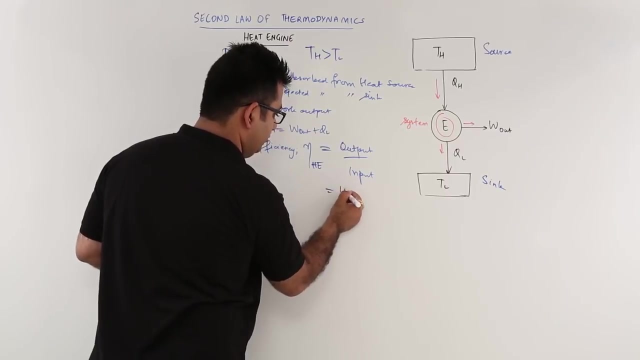 So now this gives rise to the heat engine efficiency, And that is eta, And this is eta, HE, which denotes the heat engine efficiency. Now, efficiency is basically output upon input. Now, output, in this case is W out, Ok, And input in this case is the heat input from TH. 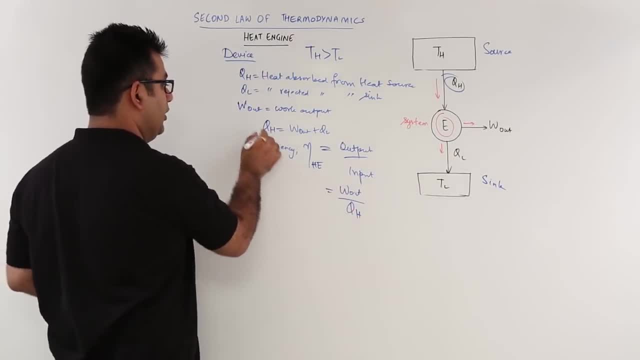 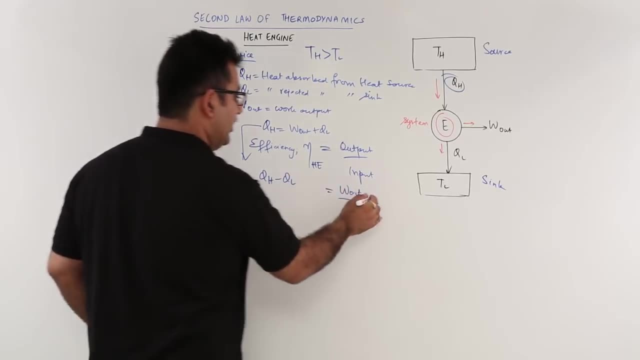 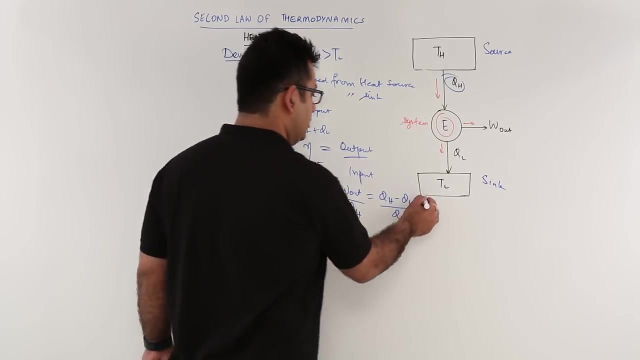 So QH. So if you replace the value of W out, So W out from this equation becomes QH minus QL. So you put it there: It becomes QH minus QL upon QH. Ok, So this gives rise to 1 minus QL upon QH. 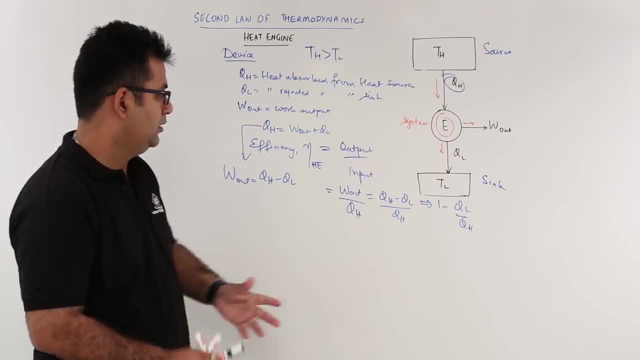 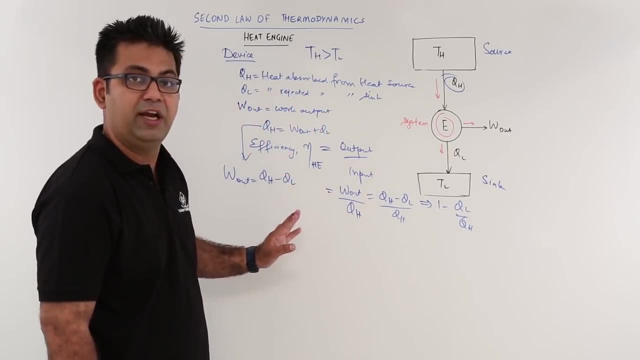 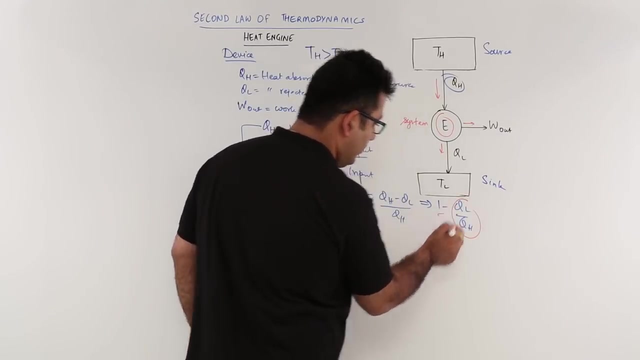 Ok, So this is the mathematical relation for the efficiency of a heat engine. Now it clearly shows that the efficiency of the heat engine is always less than 1.. Because you are subtracting some fraction from unity. Ok, So this entire value will be less than 1.. 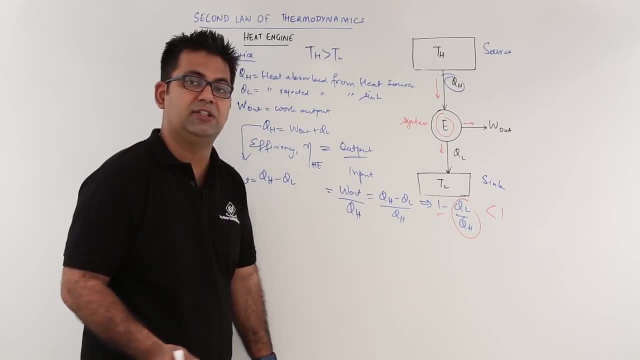 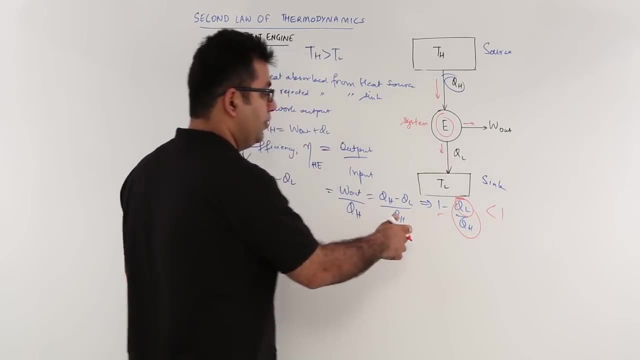 Ok, Now to make it equal to 1. that is 100% efficiency. You would have to reduce QL. Either you reduce QL or reduce it to 0, which is not possible at all. You can only possibly increase QH. 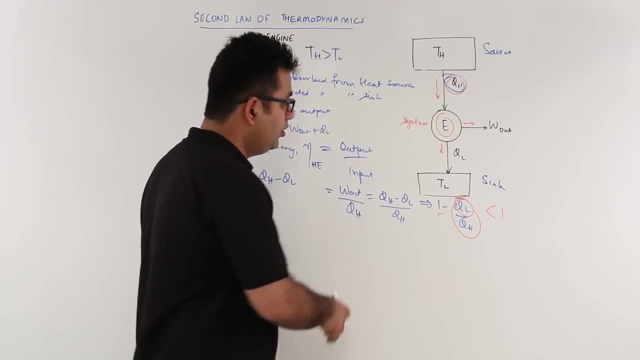 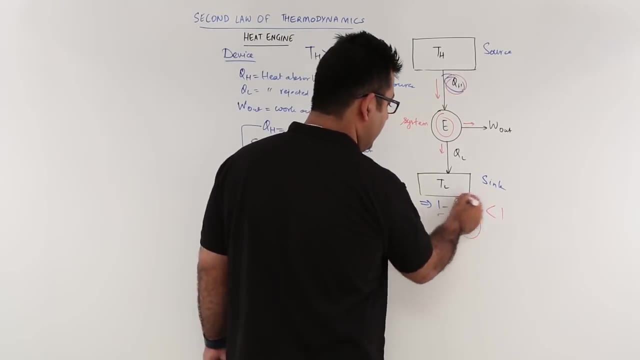 Ok, So by increasing QH, then only you can increase your efficiency, which is close to 100%. To make it exactly equal to 100%, you will have to reduce QL to 0, which is not possible at all, Because there are two things. 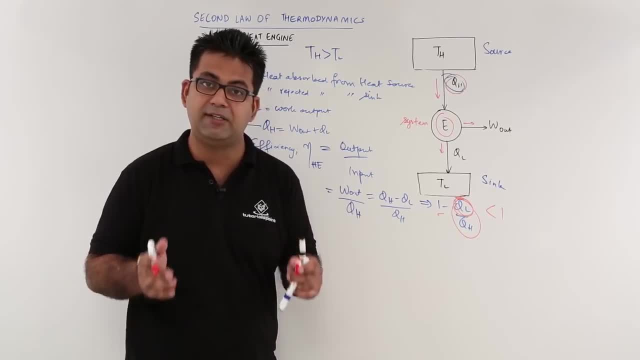 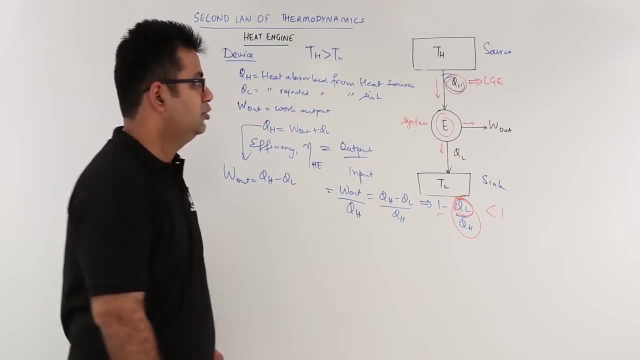 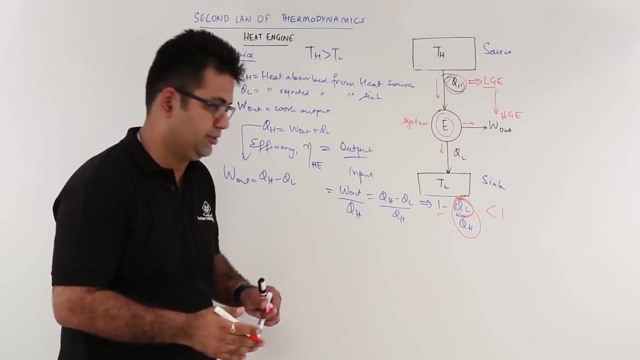 Nothing in this world is efficient 100%. Secondly, this is heat, And heat is a low grade energy. Ok, So this low grade energy cannot fully convert into a high grade energy, So this is also one of the limitations. Ok, So this is a brief introduction on the topic of heat engine. 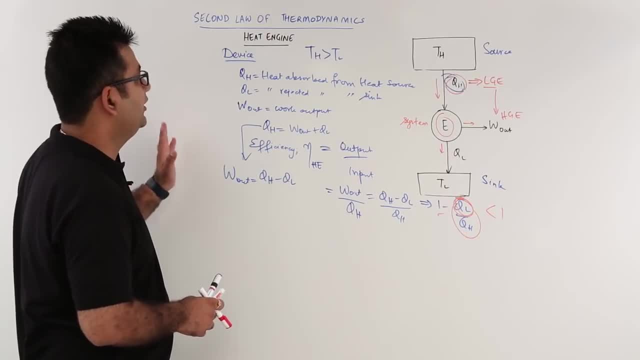 I hope you understood this. Now let's move forward from heat engine and talk about a heat pump and a refrigerator.